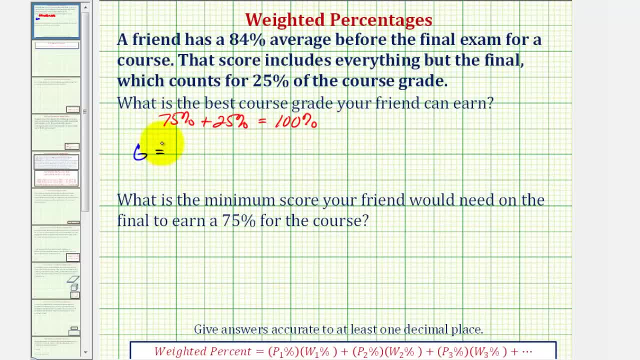 So, going back to our question, your friend's grade is going to be equal to the current average of eighty-four percent as a decimal. zero point eight. four times the weight of seventy-five percent as a decimal, that would be zero point seven five. 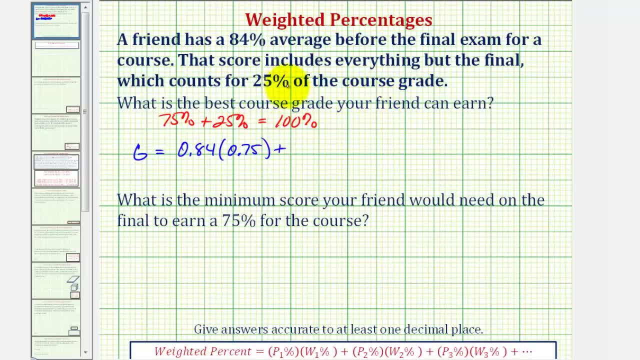 plus the best score on the final, which would be one hundred percent as a decimal, that would be one or one point zero, zero, if that's helpful times. the weight of twenty-five percent as a decimal, zero point two, five, The sum of this product would be: 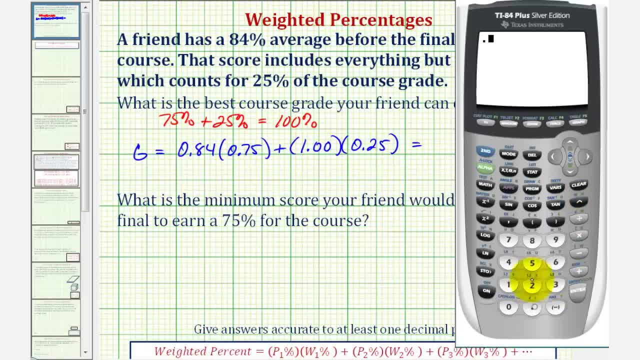 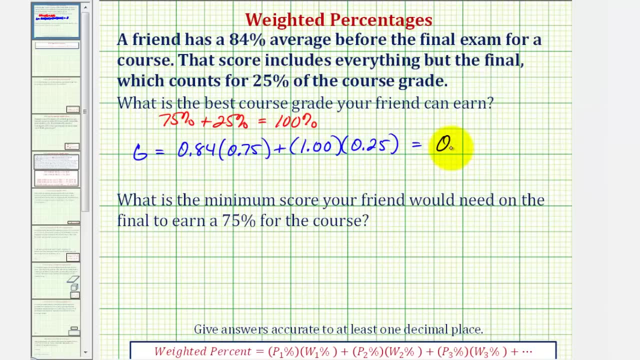 the best possible course grade. So we have point eight four times point seven, five plus well, one times point two. five is just point two five. So this gives us zero point eight, eight. As a percentage, this would be eighty-eight percent. 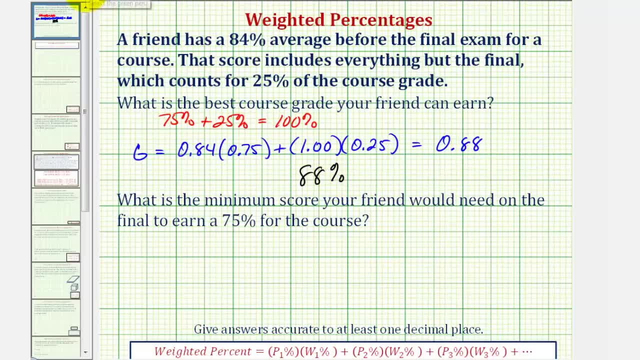 We multiply by one hundred and add the percent sign. So the best possible course grade for your friend would be eighty-eight percent. Next, what is the minimum score your friend would need on the final to earn a seventy-five percent for the course? Notice here that seventy-five percent. 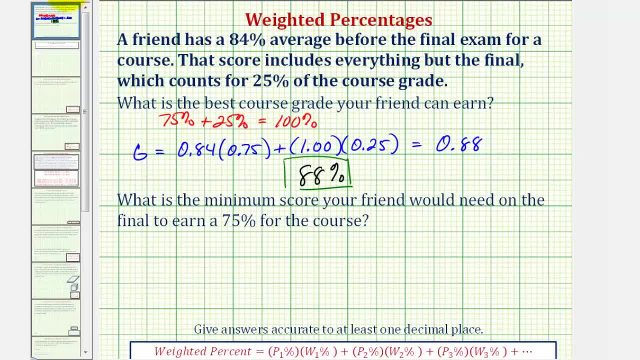 would be the overall grade or g. So we'll set this up as an equation. We'll have zero point seven. five must equal again the current average times seventy-five percent or zero point eight, four times zero point seven five. 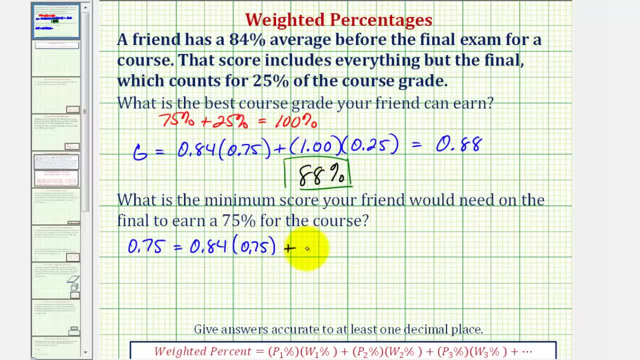 plus. now we have an unknown final exam score, which we'll call x times zero, point two, five, the weight of the final. So if we solve this equation for x, we can determine the minimum score needed to earn seventy-five percent for the course. 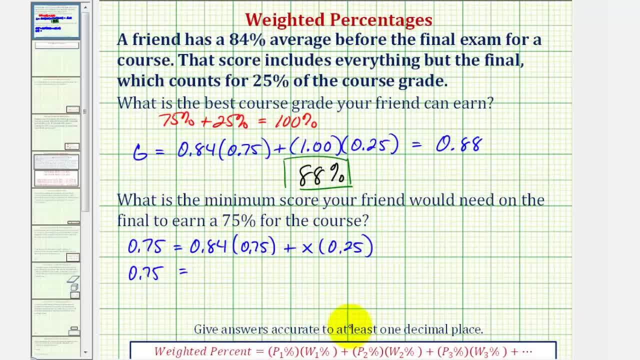 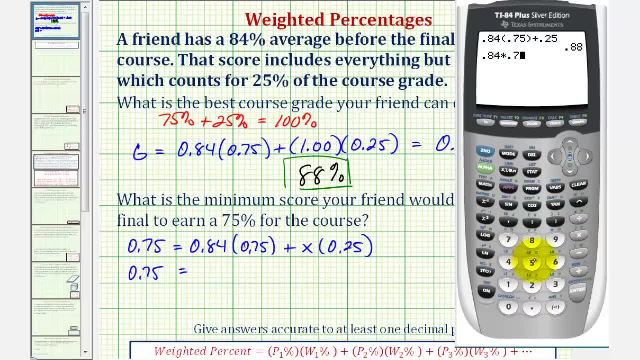 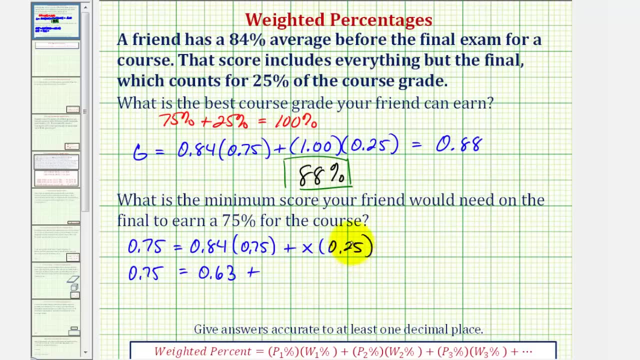 So we have zero point seven. five equals zero point eight, four times zero point seven, five, which gives us zero point six. three plus x times zero point two. five is zero point two five x, which is the total To solve this for x.